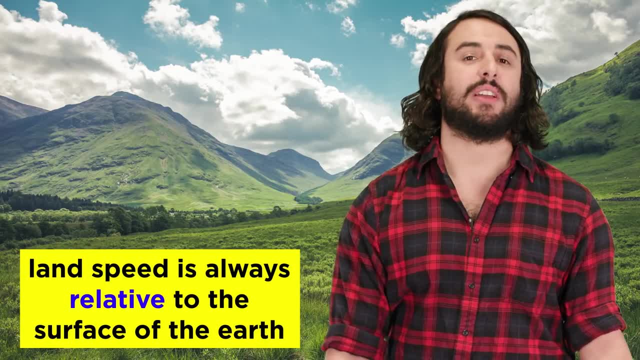 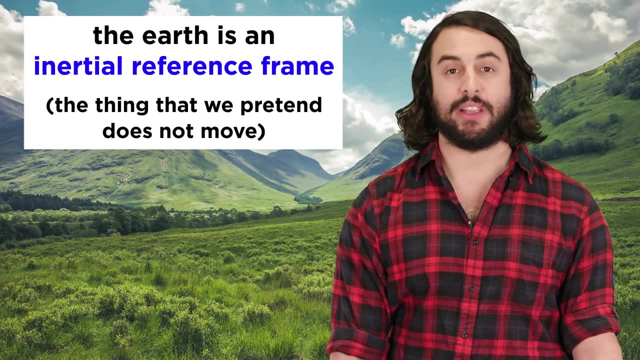 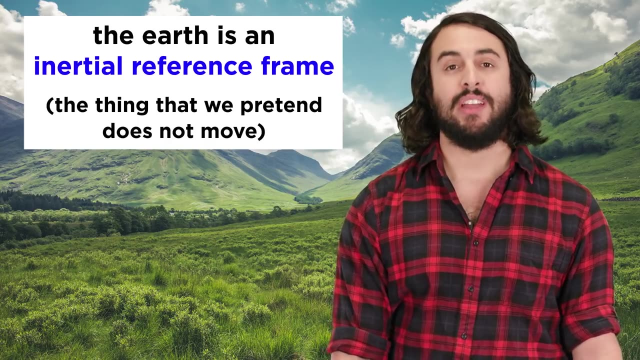 ready to pull you over. So we often discuss motion that is relative to the surface of the Earth. When we do this, we are assigning something called an inertial reference frame. This is the object or person or location that we pretend is completely still and we 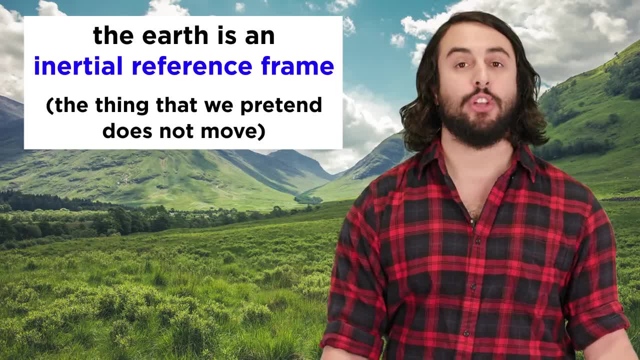 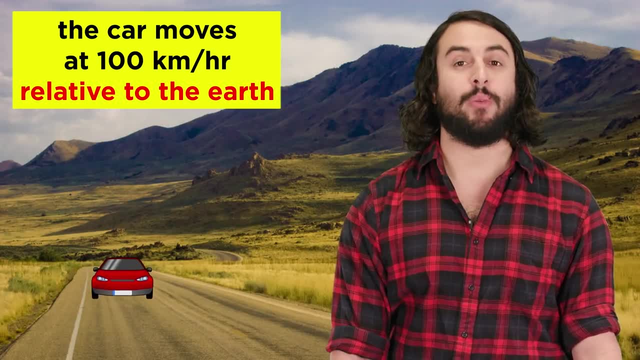 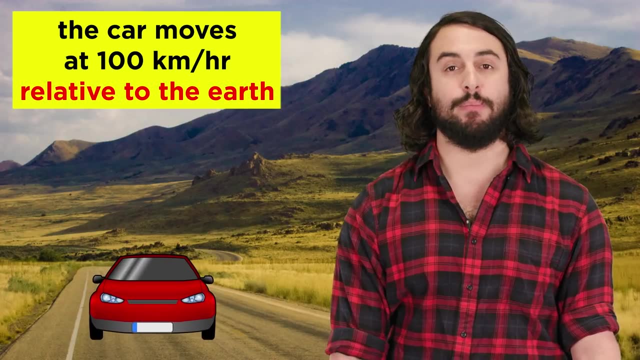 assess the motion of other objects relative to this inertial reference frame. For example, if we treat the Earth as an inertial reference frame and we ignore its rotation and movement through space, it becomes meaningful to say that this car is moving directly north at 100 kilometers per hour. 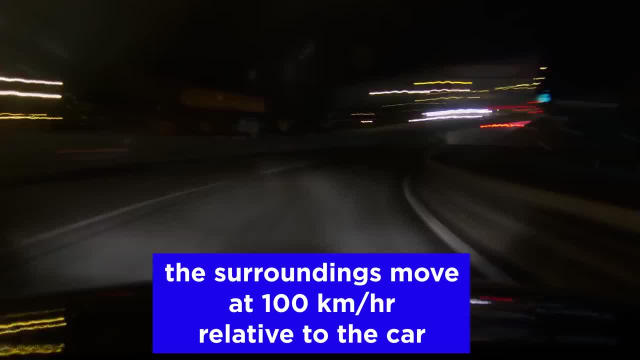 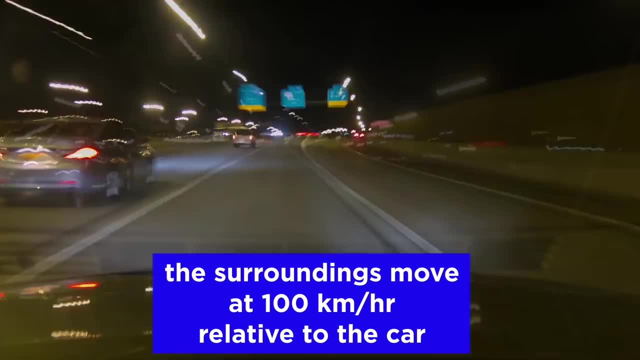 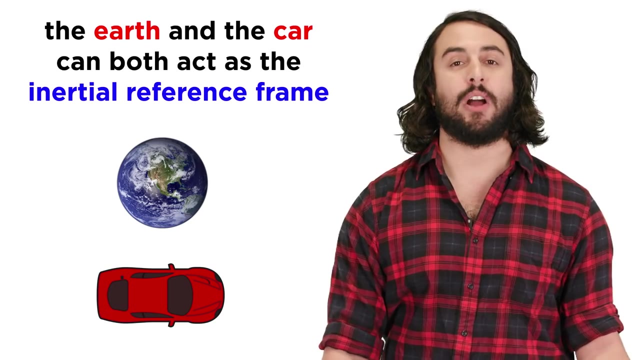 relative to the ground. But if we are inside the car moving with constant velocity, it seems as though we are not moving, but rather that the surroundings are rushing past us at 100 kilometers per hour. The car has become the inertial reference frame that is standing still. 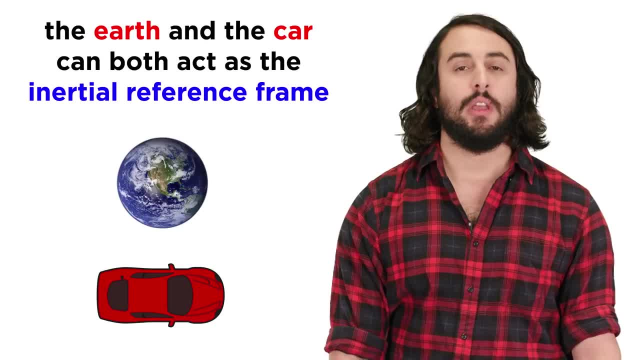 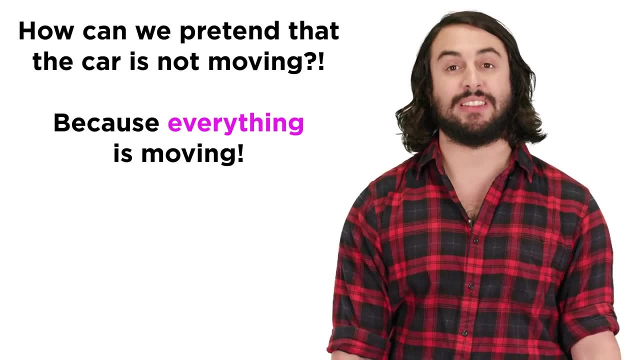 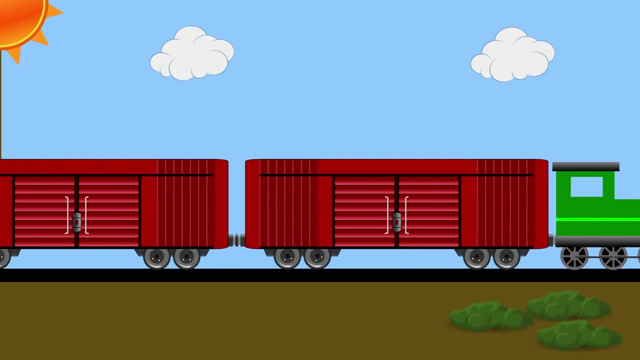 and everything is in motion around us. It may seem strange to pretend that the car isn't moving, but remember, it's just as incorrect to pretend that the Earth isn't moving. so it really is all relative. Imagine you are sitting in a moving train. You toss a ball into the 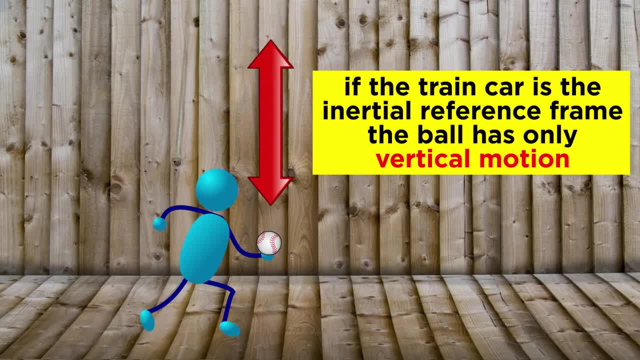 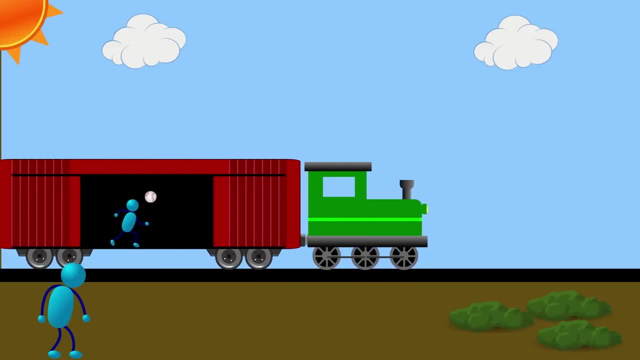 air and catch it. To you, the ball went straight up and down, but to an observer on the ground, the ball followed a parabolic path as the train went past. This is because when the ball leaves your hand, it still has all of the 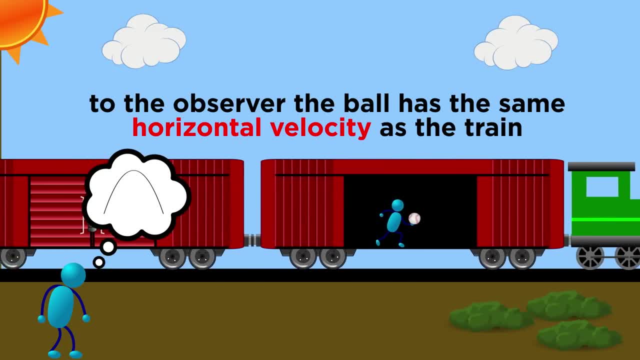 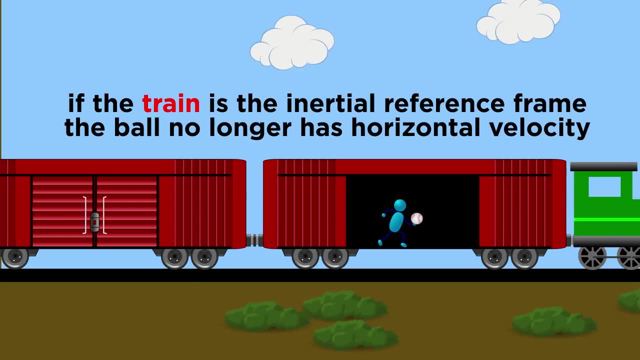 forward velocity. that the train does. But if you are inside the inertial reference frame of the train, the train is not moving at all. It is the surroundings that are moving. so the ball no longer has any horizontal velocity, only the vertical velocity you impart to. 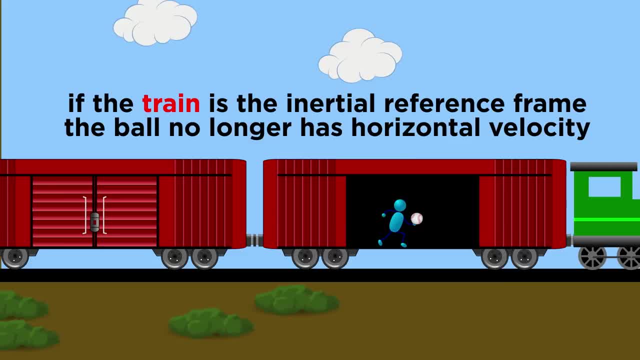 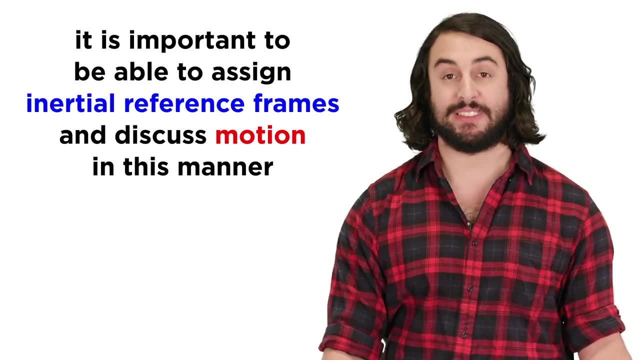 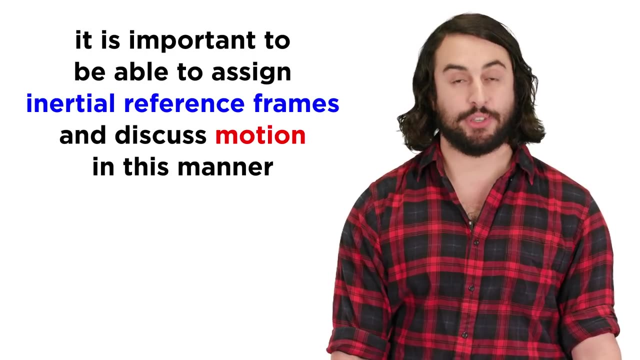 it by moving your arm to throw the ball. Assigning frames of reference and understanding what they mean for the motion of objects is a big part of physics, and although some aspects of this kind of thinking seem obvious, they were not always well understood. 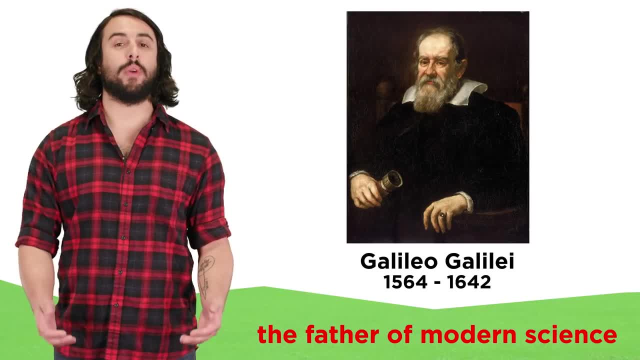 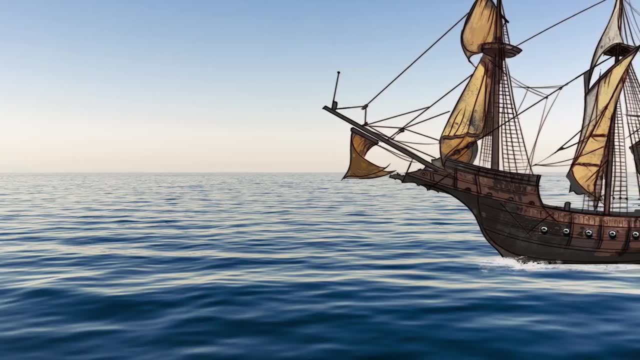 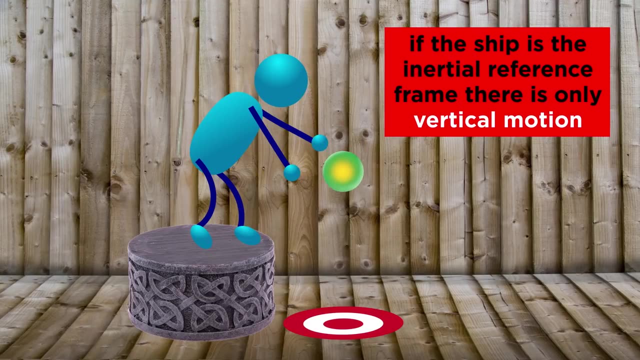 Galileo was the first to rigorously describe relative motion. after doing experiments in a moving ship, He found that if he dropped a ball while the ship was moving with constant velocity, it fell straight down, just like it did when the ship was stationary in the port. He then 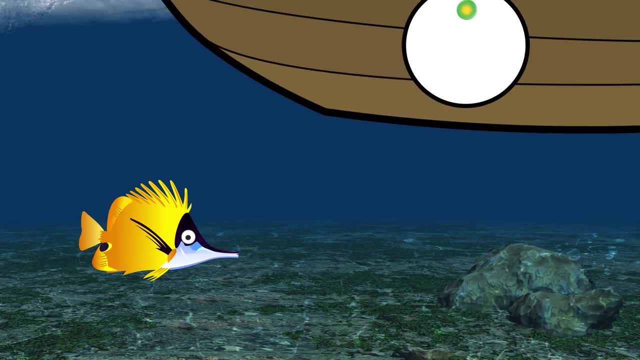 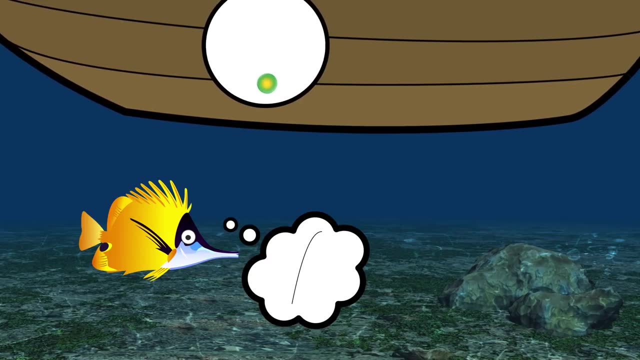 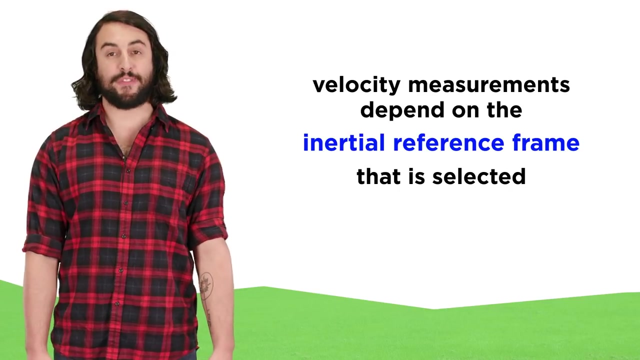 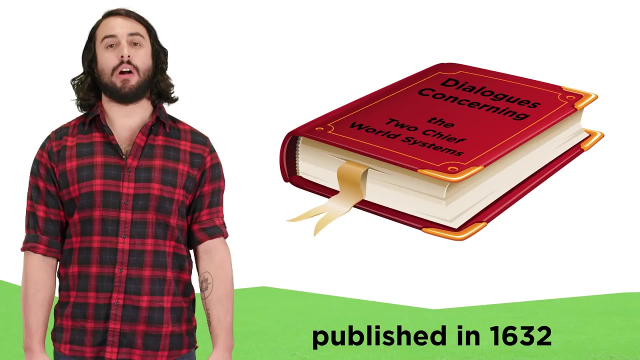 contemplated how a fish nearby would view the motion, with the ball moving forward as it falls, and how this differs from his own experience. He used these experiments to prove that velocity measurements depend on which reference frame you adopt, and he published his findings in a book called Dialogues. 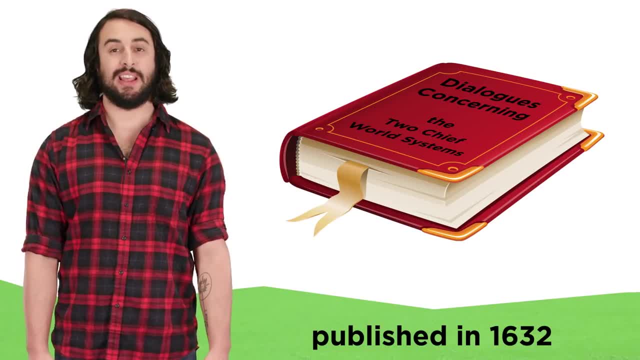 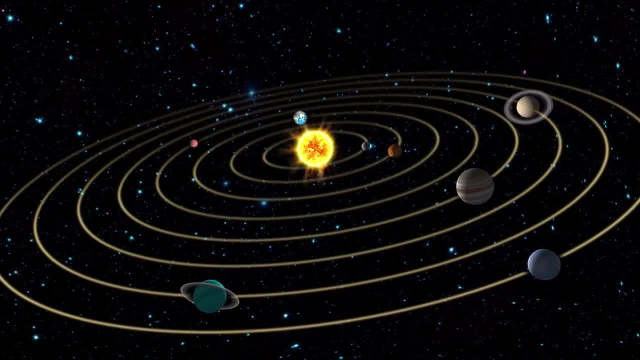 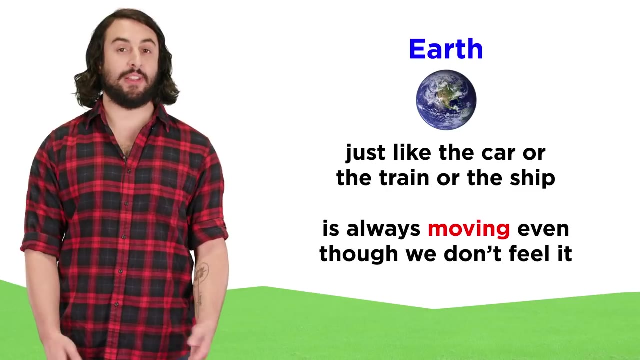 Concerning the Two Chief World Systems in 1632.. These ideas were extended to describe the motion of the earth around the Sun instead of the other way around. by proving that the earth could be moving even if we don't feel it, This got. 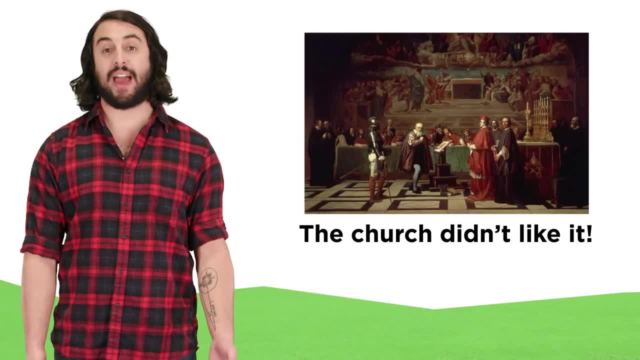 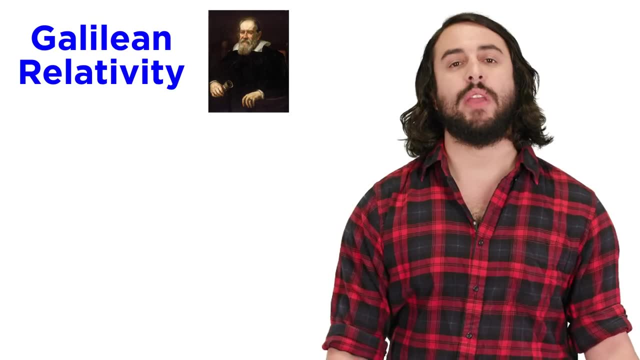 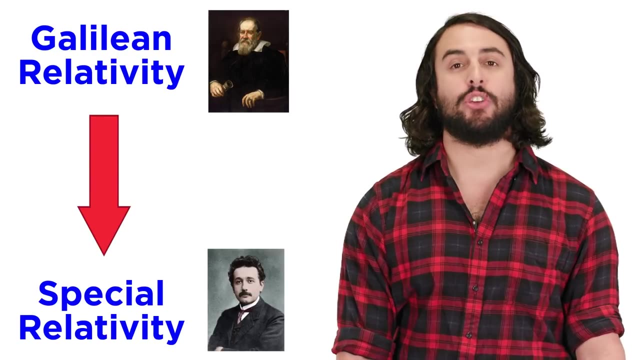 Galileo and other scientists into hot water with the Catholic Church, but humanity eventually caught up to his revolutionary thinking. We refer to this portion of his work as Galilean relativity, and these concepts are the basic set of rules that will be built. 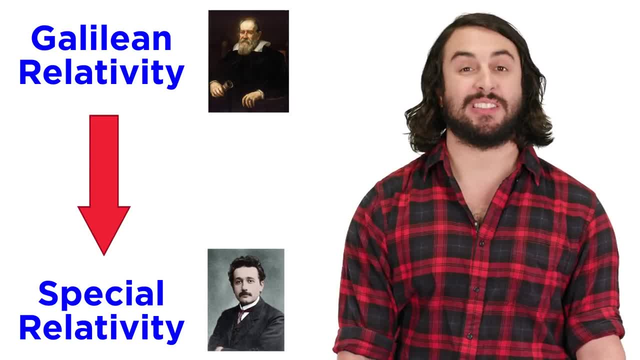 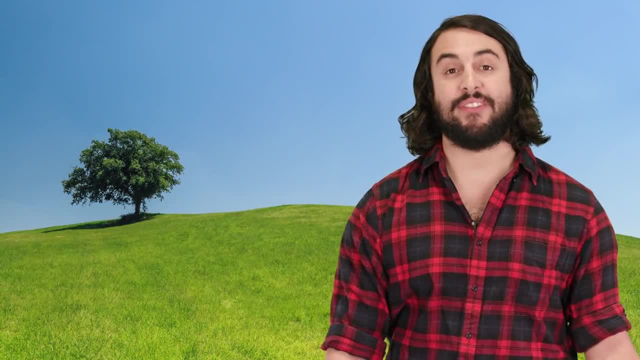 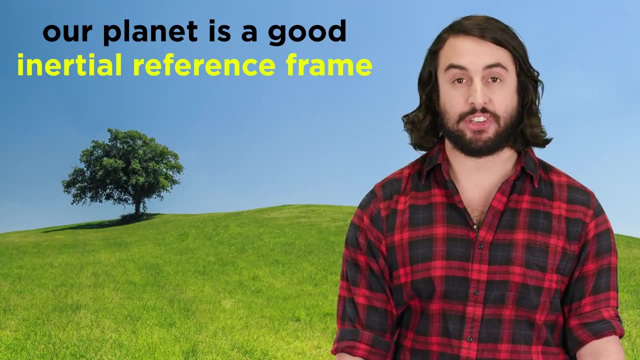 upon to enter very strange territory when we cover Einstein's special relativity in the modern physics course. But for right now we won't go flying through space. We have much more work to do on earth which, despite its rotation and motion, is actually quite a good. 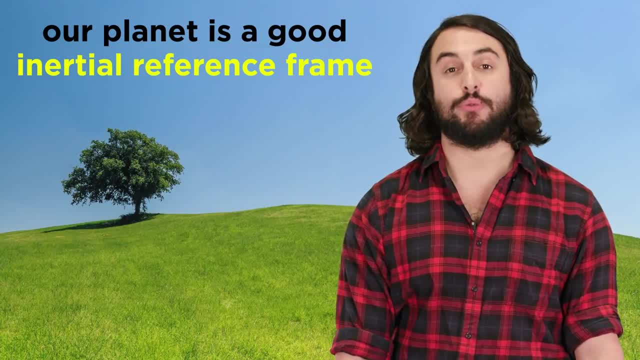 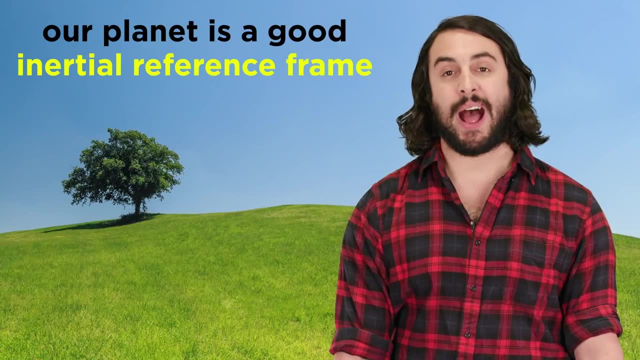 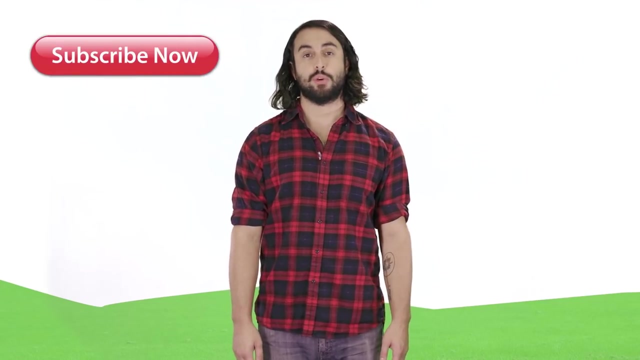 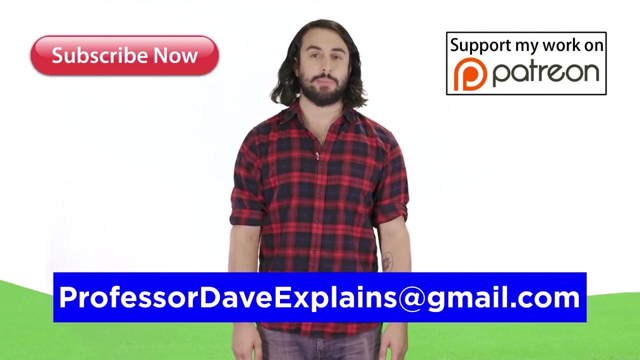 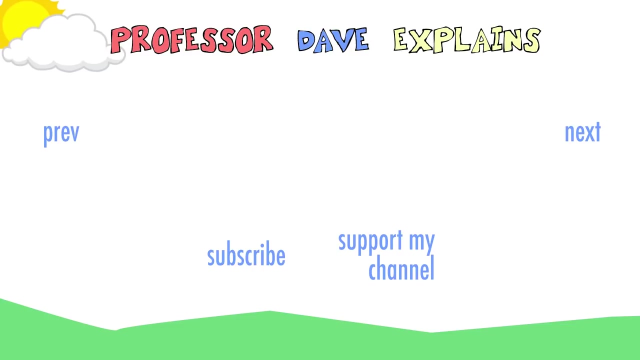 approximation of an inertial reference frame, one that will be used frequently throughout our study of physics. With each topic we go through, whenever we are, Whenever we examine an object's velocity, just remember it's all relative. © transcript: Emily Beynon.